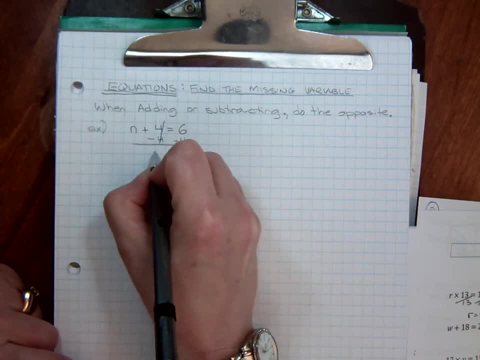 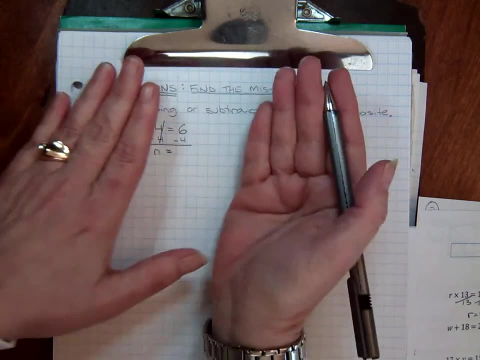 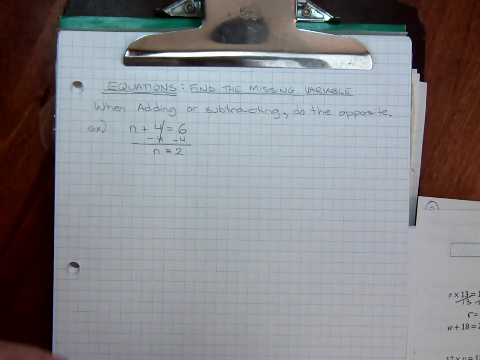 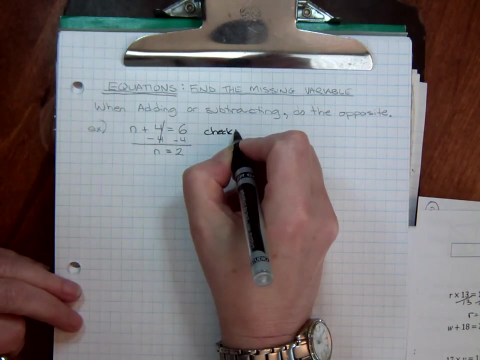 4 minus 4 is 0. So there's nothing left there. N is finally by himself. That's what I wanted On this side of the equal sign. Okay, we've got N On this side of the equal sign. I've got: 6 minus 4 is 2.. Now, if I want to check that, I can do a check That will help me. I said that N is 2.. So where N is, I'm going to substitute in the number 2.. 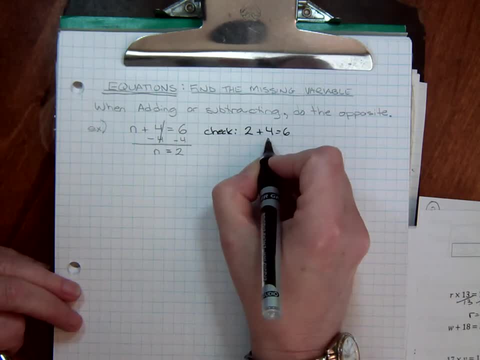 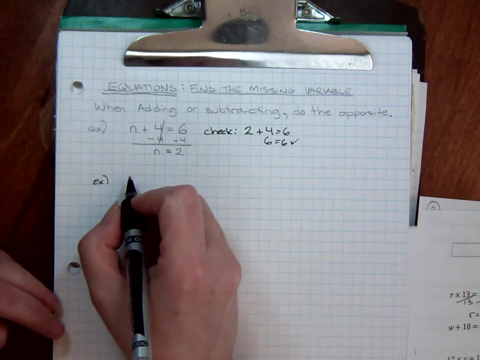 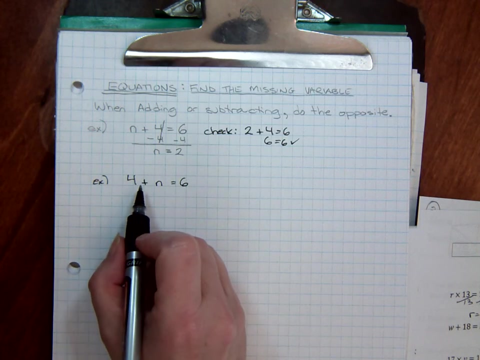 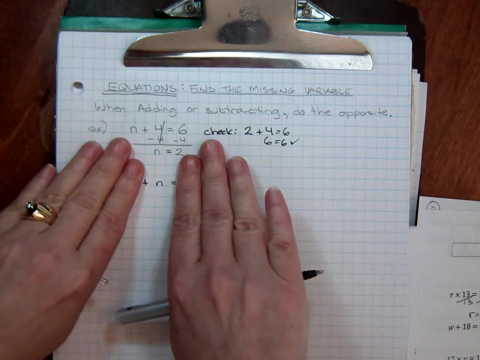 So 2 plus 4 equals 6.. 6 does equal 6.. I did it right. Okay, let's do another one. Let's change the order this time. What if I have 4 plus N equals 6? This is still an adding question. Now, over here I've got to get this 4 onto this side of the equal sign. That's the goal: To isolate N all by himself. So to get rid of this. 4, it's a positive 4.. It doesn't say that. But if it's a positive 4, it's a negative 4.. 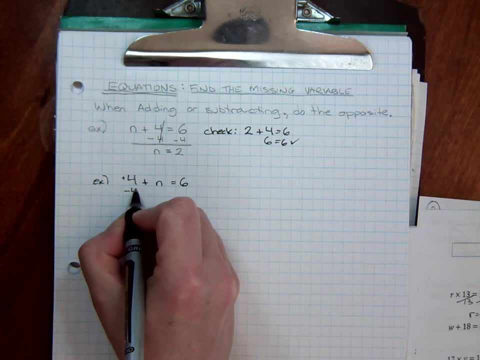 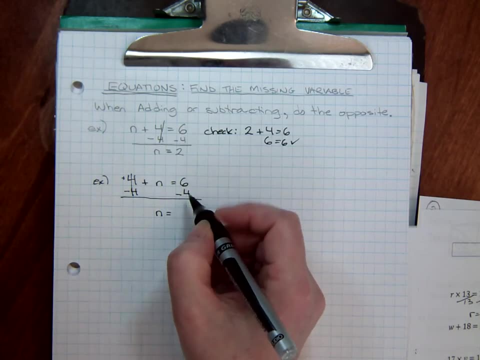 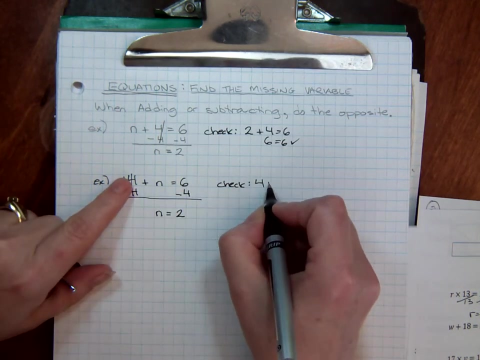 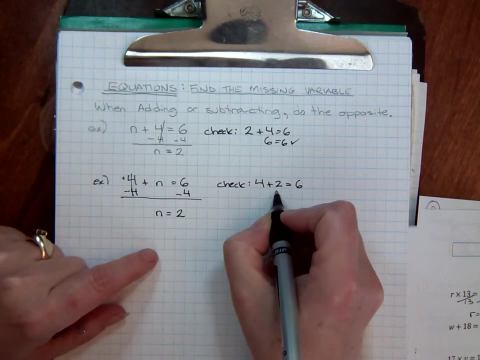 It's invisible, It's 4.. It's positive. I will subtract 4 from both sides. These cancel: N is by himself. 6 subtract 4 is 2.. And if I want to check it, I will go 4 plus. now I said N is 2.. So instead of N I'm going to write 2 equals 6.. 6 does equal 6.. I did it right. Let's do some subtracting ones. 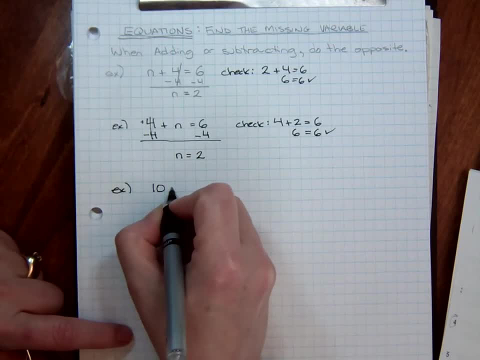 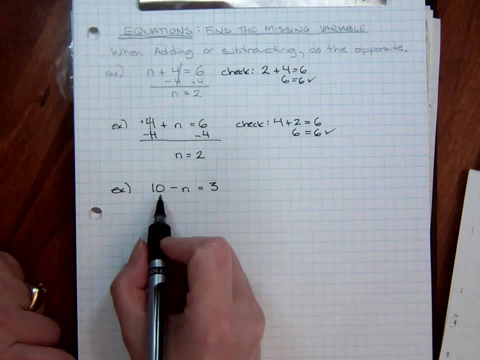 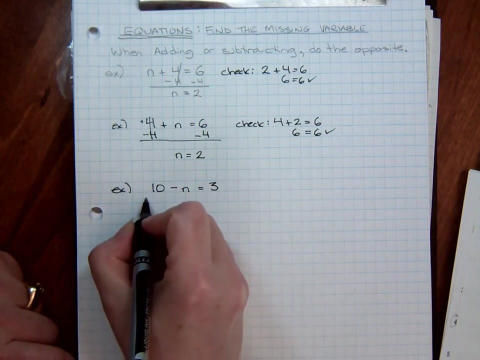 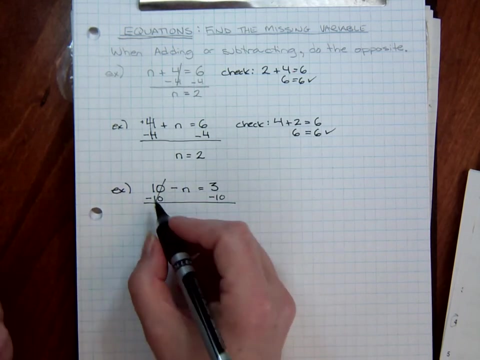 Okay, what if I have 10 minus something equals 3? Well, this is a tough one. The negative N, But still I've got a positive 10 over here To get rid of him, to get him to go to the other side to get rid of a positive 10, I will subtract 10.. Okay, these cancel Because 10 minus 10 is nothing. So there's nothing there, But I've still. now I've got a negative N equals 3 minus 6.. 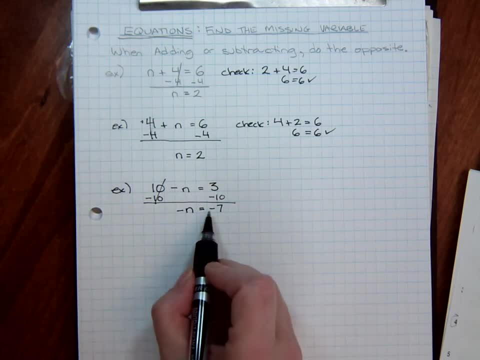 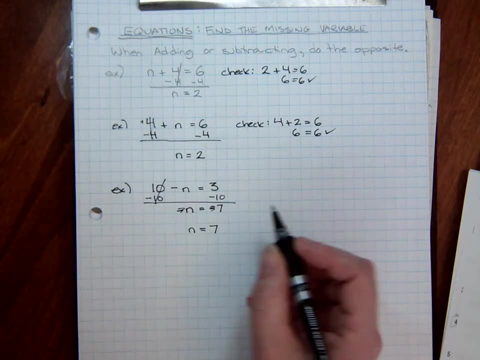 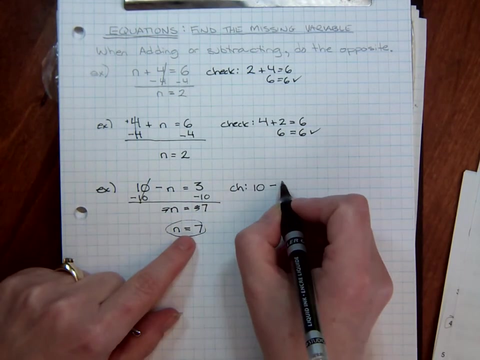 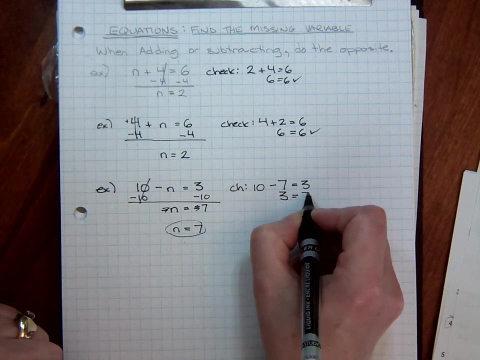 10 minus 10 is negative 7.. When both of these are negative, they just cancel. So N is 7.. Just cross them out. Okay, now I can check it. if I want, Let's check it. 10 minus 7, because I said N is 7, equals 3.. 10 minus 7 is 3.. So 3 does equal 3.. I did it right. Let's do another one. 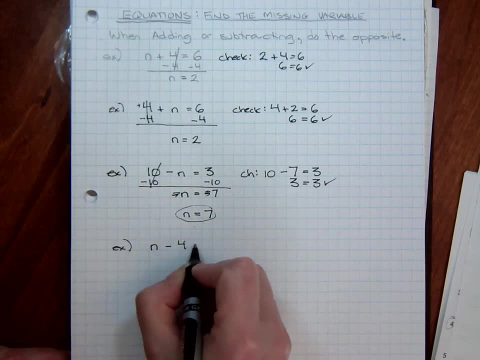 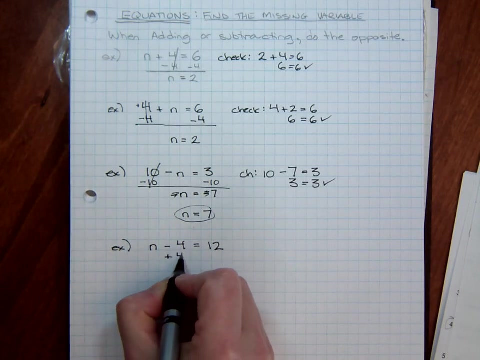 What if I have N minus 4 equals 12?. So here's what I do in my head: Something minus 4 equals 12.. So something subtract 4 is 12.. This is a negative 4.. To get rid of a negative, I do the opposite: I add 4.. Negative 4 and a positive 4, they cancel. N is by himself, That's what we wanted, And it equals 12 plus 4, which is 16.. 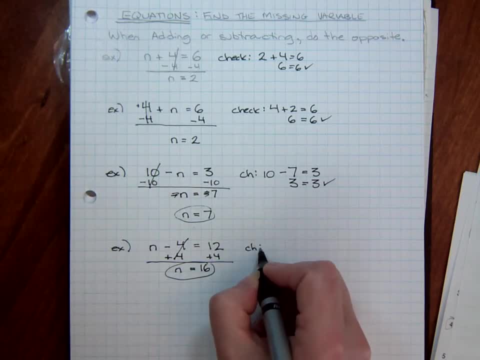 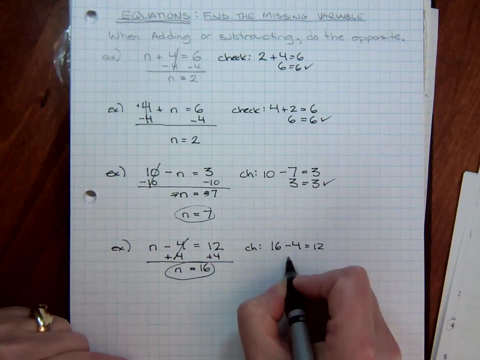 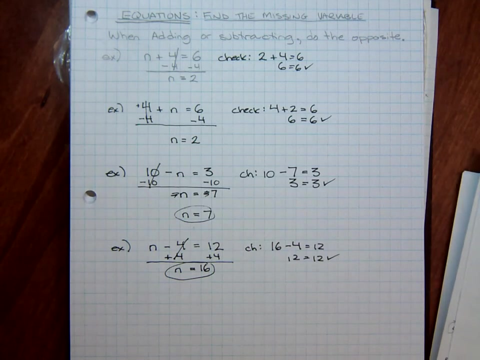 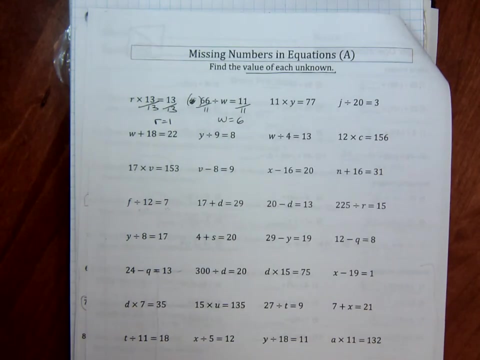 Now I can check that. I said N is 16, so I'll substitute that in 16 minus 4 equals 12.. 12 does equal 12.. So we did it right. Okay, now let's try and do some of the problems from missing numbers in equations A. Find the value of each unknown. 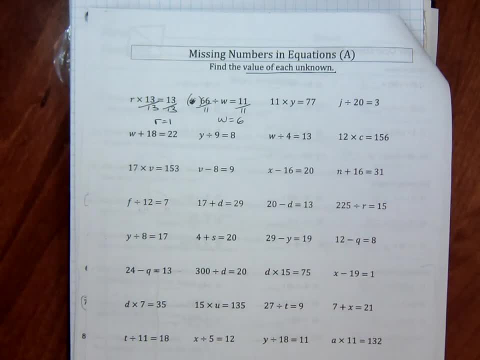 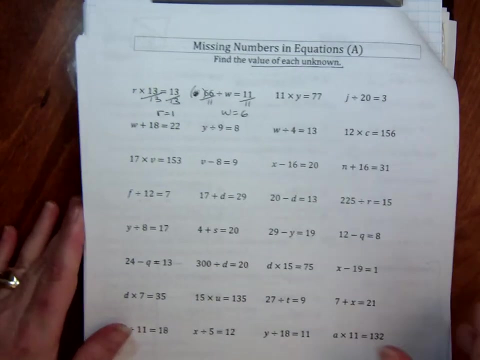 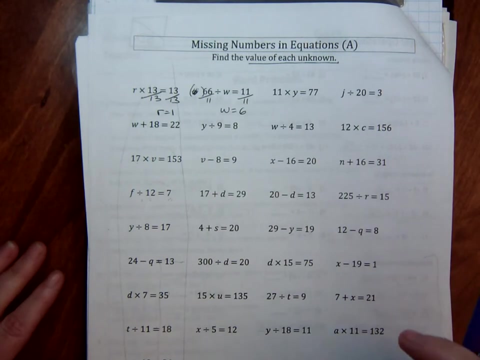 Hold on a second. Let me get a better pencil here. All right, and we're back. Okay, let's start. I'm going to do this whole first column with you and then I'll leave you to the other three. You can take a picture of them and send it to me. 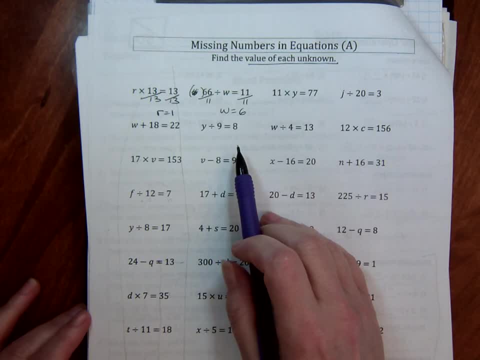 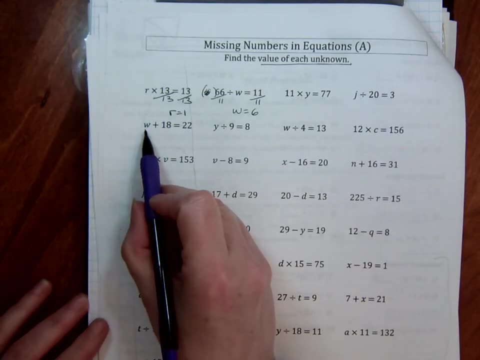 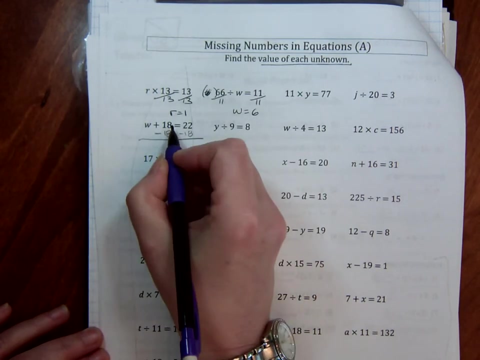 Or, if you want, there's a package in my mailbox at school, And if you don't have that, you can just write these all down on a piece of paper. Okay, Okay, something plus 18 equals 22.. I'm going to subtract 18 from both sides. These cancel And W equals 4.. 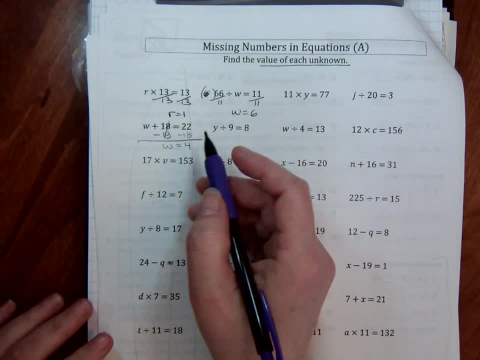 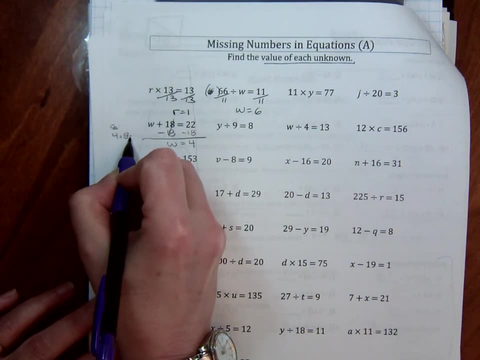 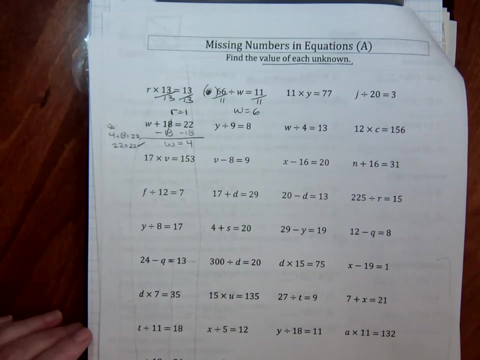 I can check it if I like. You can check it on your own. The check would look like this. I'm going to write really small: 4 plus 18 equals 22.. 22 does equal 22.. Okay, so you can do the checks on a separate piece of paper. 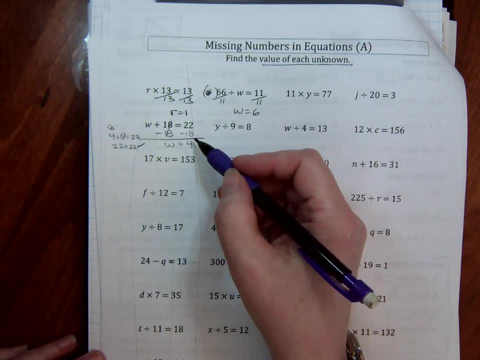 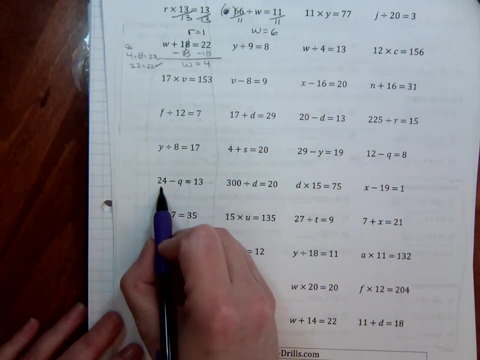 Then you'll know if you've done it right. Okay, I'm going to. let's do. let's do all the adding and subtracting ones in this column. Let's see, here's one here: 24 subtract something equals 13.. 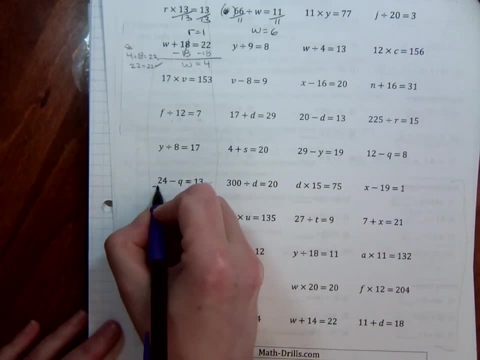 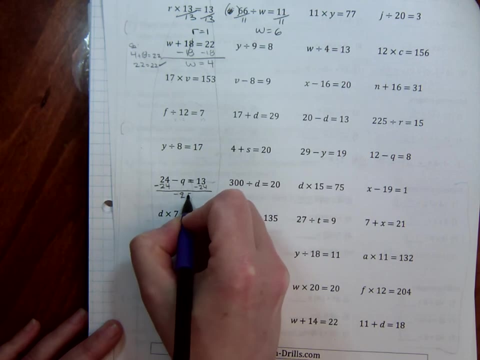 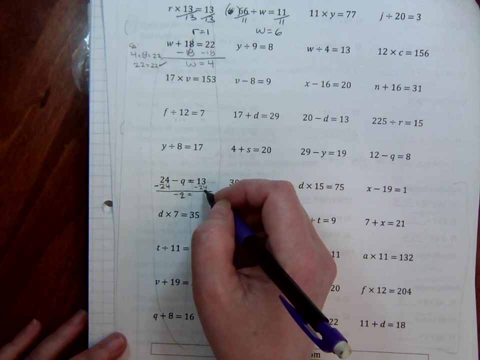 Well, this is still a positive 24.. So to get rid of it, I will subtract it from both sides. Now I've got negative Q equals. what is that? 7. 13 minus 24.. 24, 11, negative 11.. 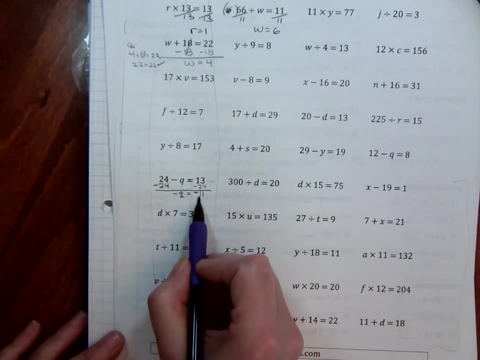 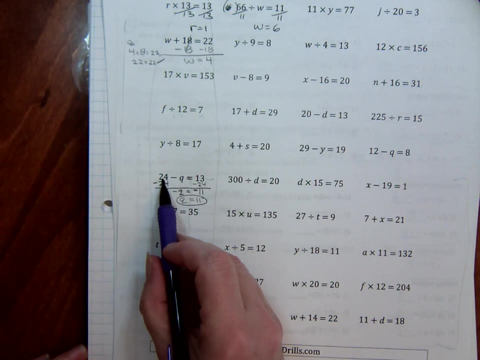 Now, since both the variable and my number is negative, it just becomes a positive. So Q equals 11. And I could check that 24 minus 11 does equal 13.. Let's see if there's any more here. Here we go. 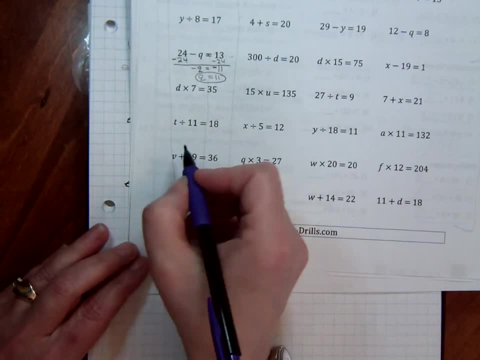 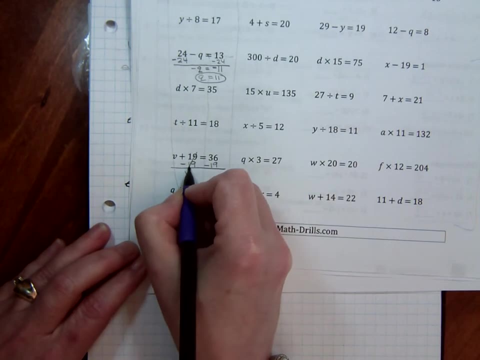 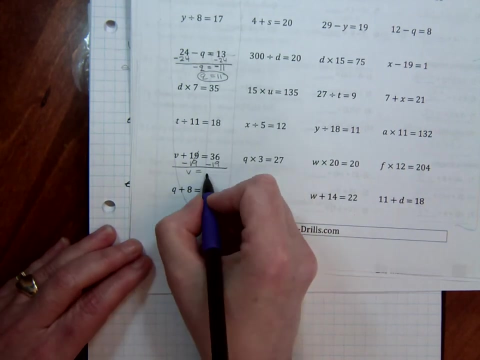 Something plus 19 equals 36.. This is a positive 19.. So to get rid of it, I will subtract: V is by himself, because these cancel. 19 minus 19 is nothing, Equals 17.. Okay, 17 plus 19 equals 36.. 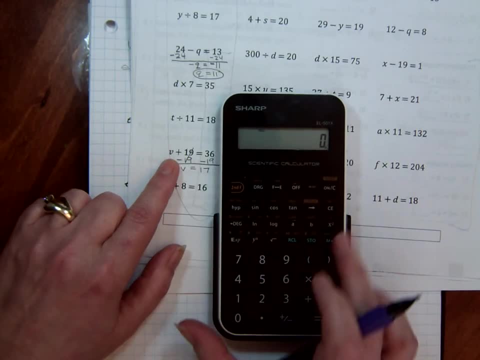 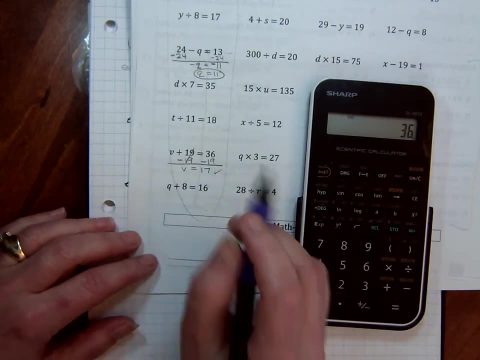 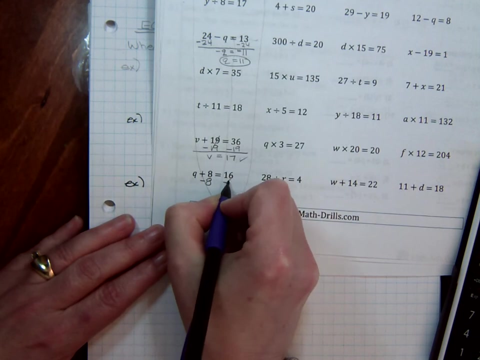 I could even check it with a calculator. I said that V is 17. So 17 plus 19, it does equal 36.. So I know it's right. One more: Something plus 8 equals 16.. I will subtract 8 from both sides. 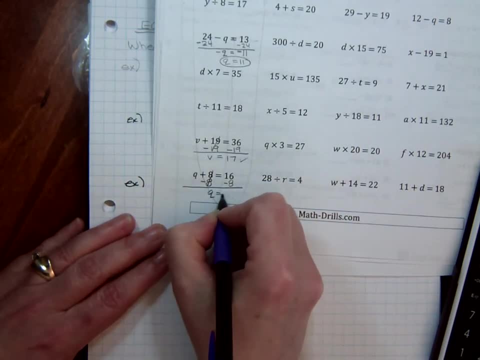 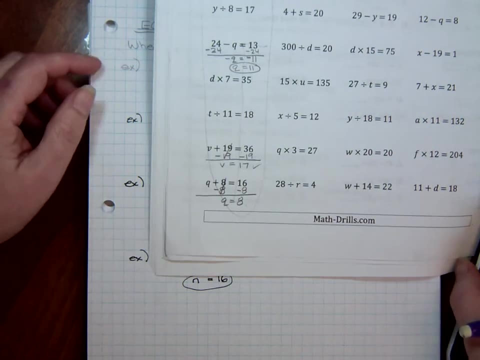 These cancel Q equals 8.. And is that true? Does 8 plus 8 equal 16?? Yes, it does. Okay, now let's take a second, go back to our notes And let's make some notes for when we're multiplying and dividing equations. 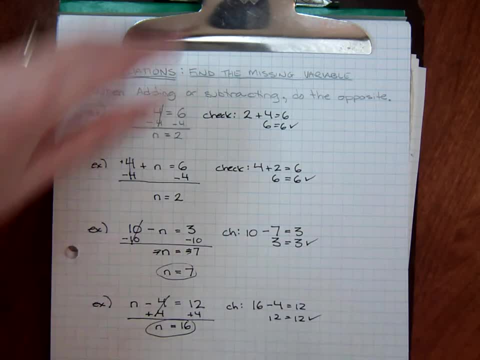 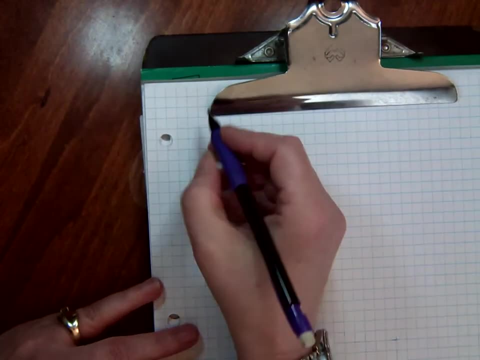 Okay, so I'm going back to the notes for adding and subtracting. I'm just going to turn my page. Oh, that marker went right through. I'll pick a new page. Now, I'll do. I'm going to do some equations when I multiply and divide. 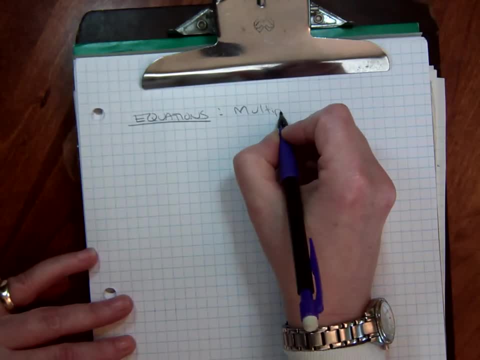 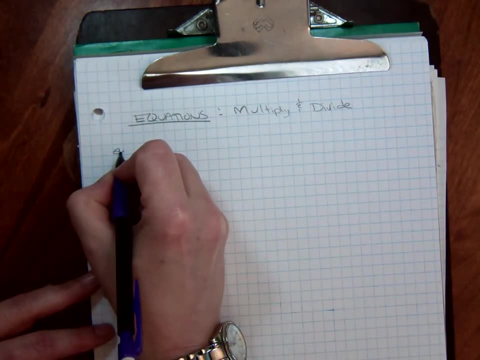 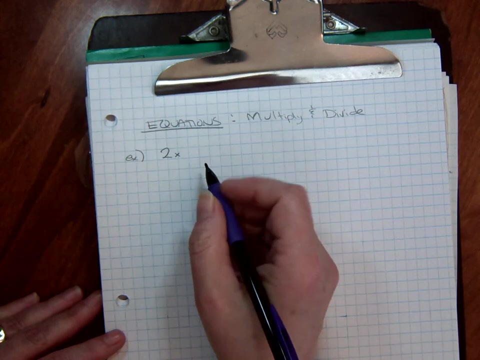 Multiply. maybe I'll write that out: Multiply and divide. Let's do some examples. Okay, let's start with multiplying. Suppose I have 2, and I hate that these sheets use X for multiply, But let's say 2 times something. 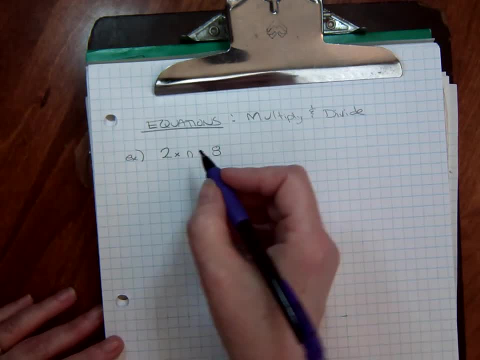 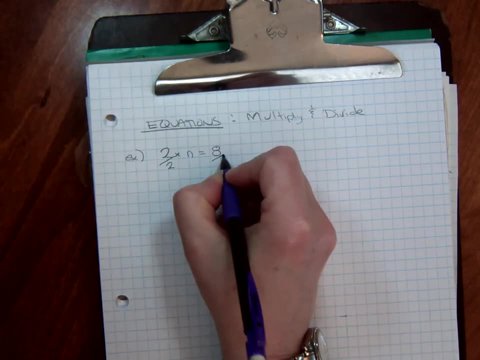 Equals 8.. In your head you probably know that's 4. But let's prove it, Okay. the opposite of multiply is divide, So I will divide both sides by 2.. 2 divided by 2 is just 1.. 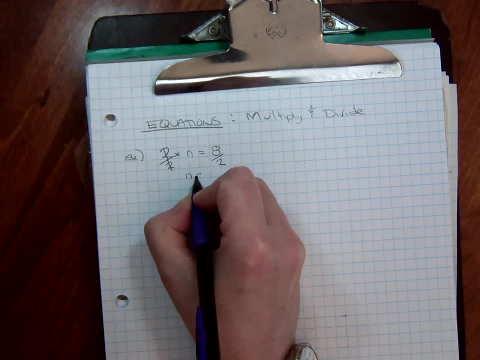 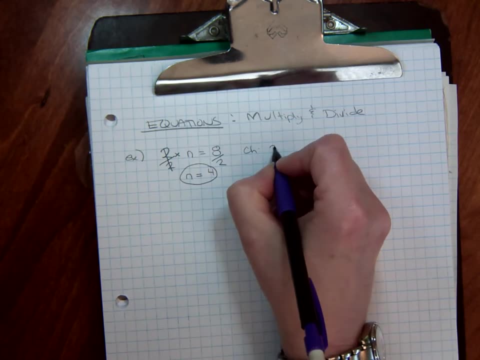 And we don't need to write a 1. It's just nothing. So N is by himself. 8 divided by 2 is 4.. If I want to check it, I will go: 2 times 4 equals 8.. 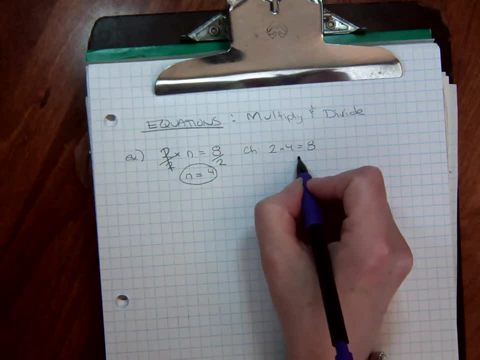 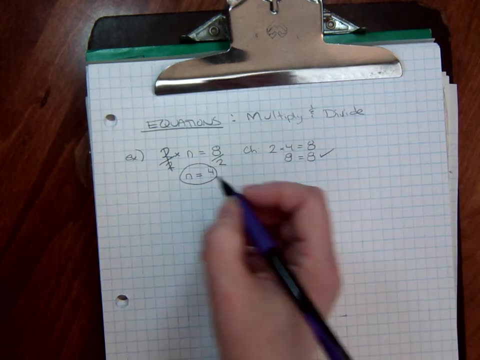 I like to check it backwards in my head to see if I'm doing it right, So I always write down the answer I'm looking for. Now, 4 times 2 is 8.. Yes, I did it right. Okay, what if they're in a different order? 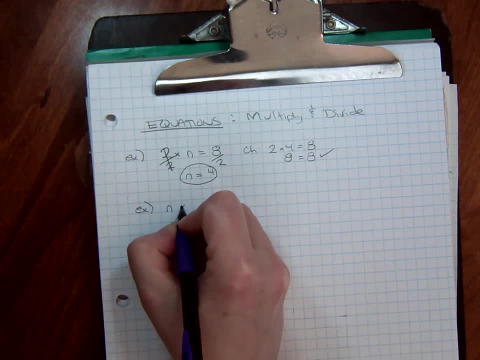 What if I had N? so something times 3 equals 15.. In your head you probably know it's 5., But let's prove it. So this is a multiplying question. The opposite of multiply is divide, So I'll divide both sides by 3.. 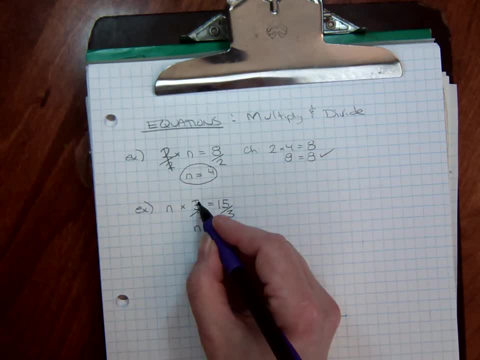 N is by himself, Because 3 divided by 3 is just 1.. N is by himself. N is by himself. N is by himself. I could write down that 1,, but I don't need to. 15 divided by 3 is 5.. 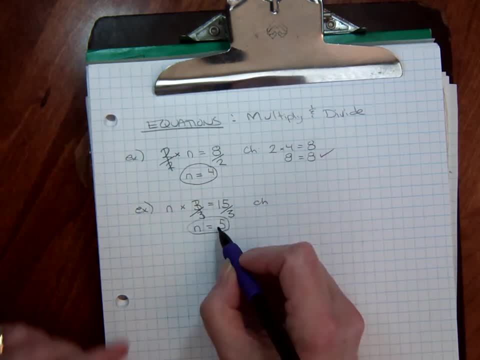 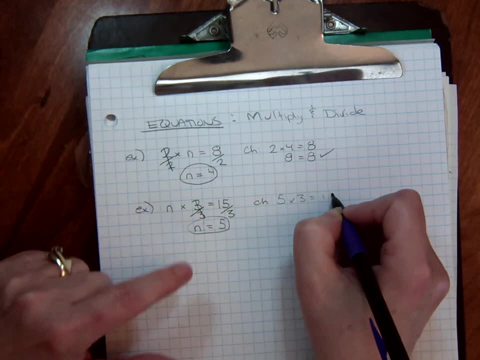 If I want to check it. I said that N is 5.. So I'm going to substitute that back in. 5 times 3 equals 15.. So the number I'm trying to find is 15.. 3 times 5 is 15.. 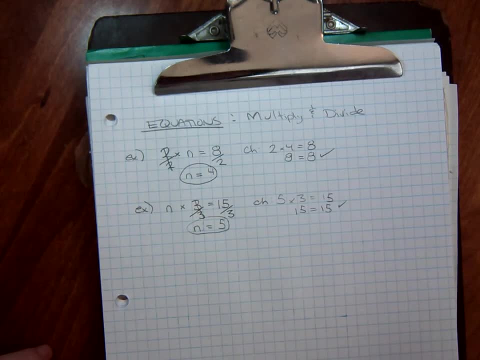 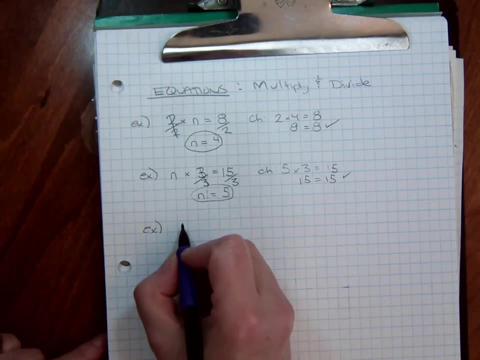 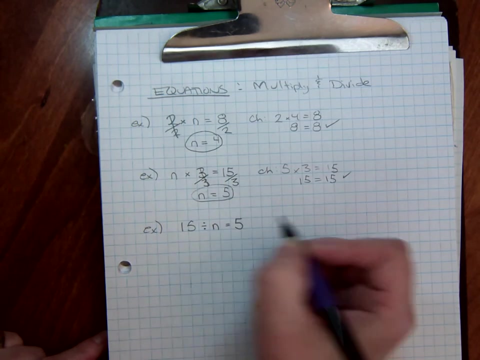 Oh, there's Mulan again. She always likes to bark when I'm online with you guys. Hi, Mulan. Okay, now let's do some dividing ones. What if I have 15 divided by something equals 5?? Now, this is the kind of case where I want you to think out loud. 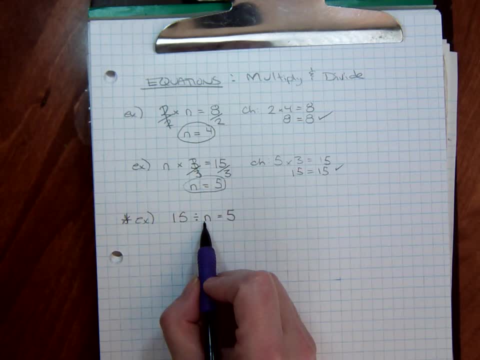 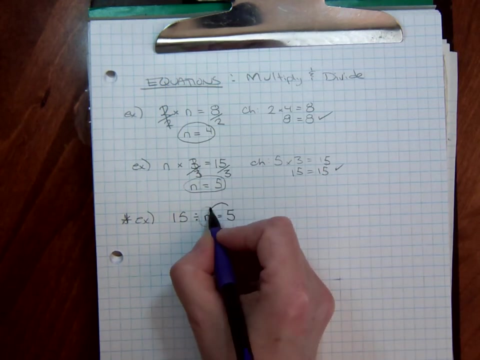 This is a thinking kind of question: 15 divided by something is 5.. Then that means that 15 divided by 5 is something. So when you see the variable set up like this, let's just switch them. okay, I want you to get used to doing that. 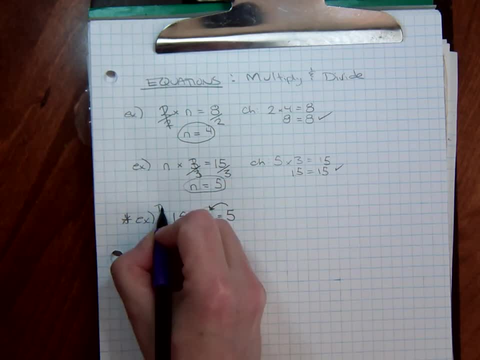 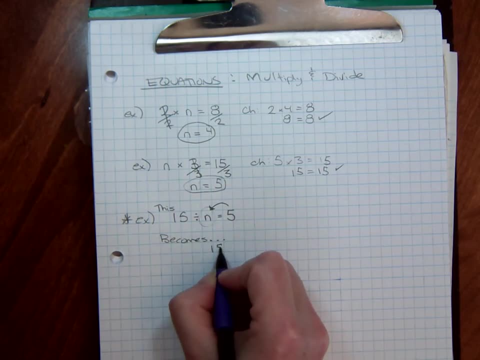 So this becomes this: 15 divided by 5 equals N. 15 divided by 5 is 3.. So N equals 3.. It doesn't matter if we wrote it backwards. I'm going to do another one like that. Okay, let's do another one. 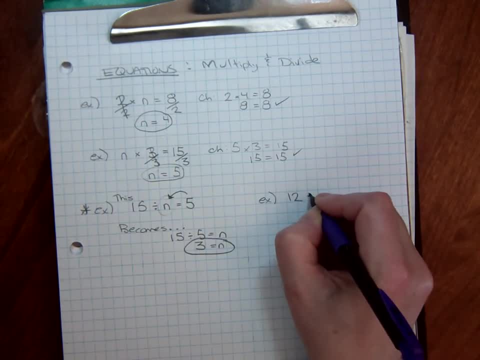 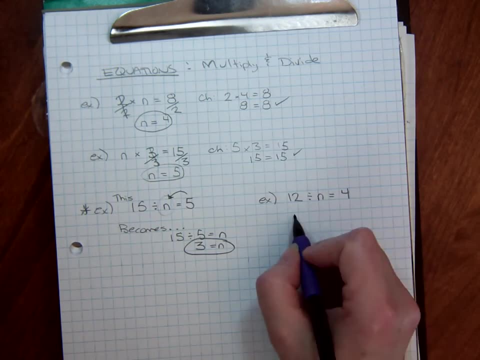 So 12 divided by something equals 4.. That also means, then, that 12 divided by 4 is something. See how we just switched these guys. Okay, so N will be 3.. Oh, how convenient. Again, not all your answers are going to be 3.. 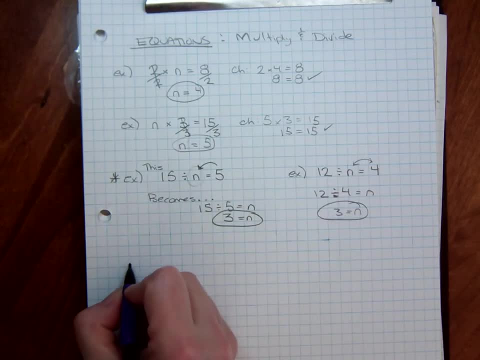 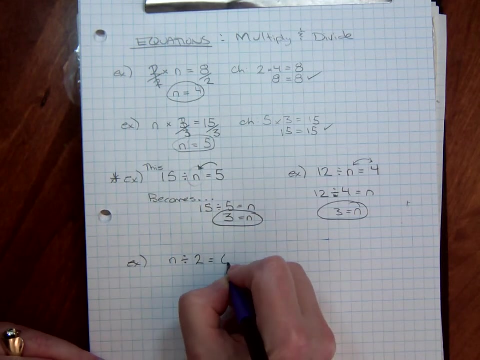 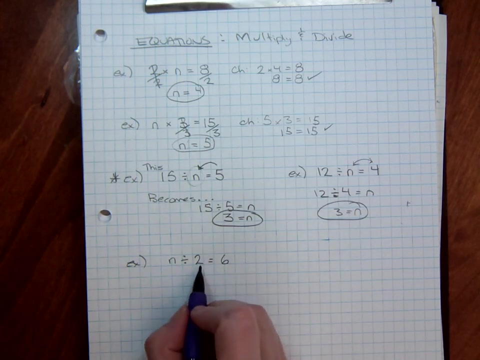 Now let's try a different kind. What if we had something divided by- what's a nice number- Divided by 2. Something divided by 2 equals 6.. So if something divided by 2 equals 6. Now, here the number is right next to the equal sign. 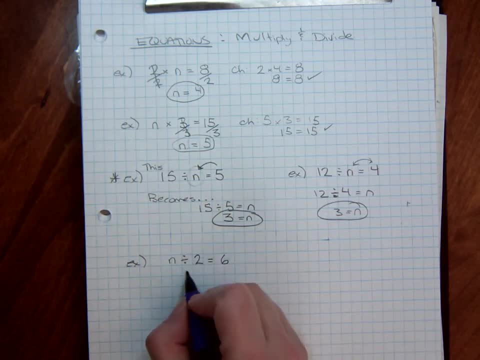 So then I could just multiply it, Because that is the opposite. So the opposite of divide is multiply. So I could multiply, Multiply both sides by 2.. I know that looks like an exponent, I didn't write that very well. Okay, these cancel. 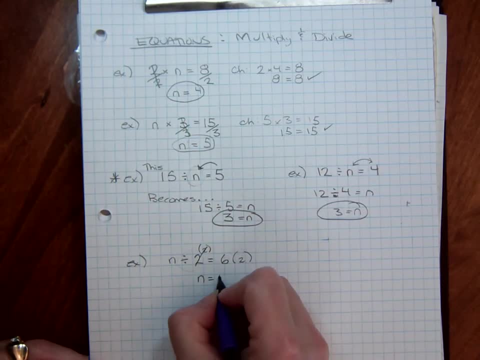 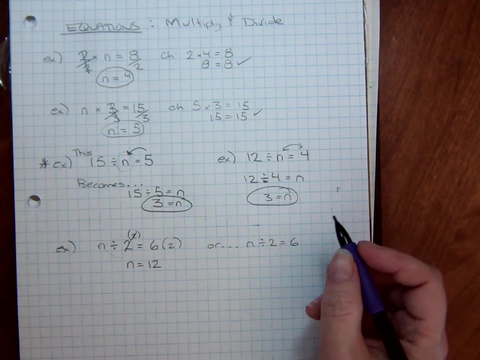 N equals 6 times 2,, which is 12.. Now another way to think about this could be okay, or you could do it this way: Something divided by 2 equals 6.. I could just flip this whole thing over. 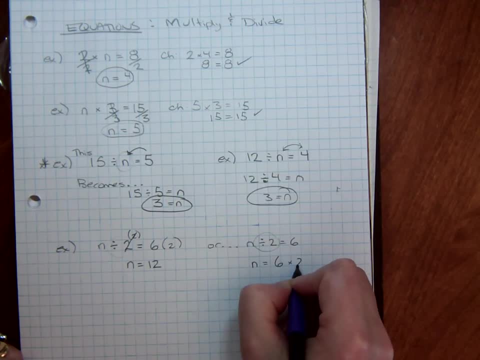 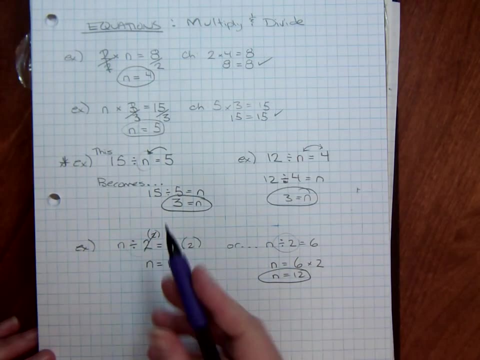 And N equals 6. Times 2.. I guess that is what we just did. It doesn't matter how your brain sees it, As long as you're doing it right. And either way, you're going to find out in the check. 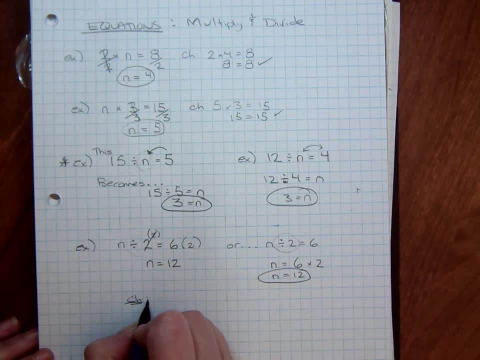 As soon as I do a check anyway, I'm going to find out. if I did it wrong, I said N is 12.. So 12, going back to my original equation. So 12 divided by 2 equals 6.. 6 does equal 6.. 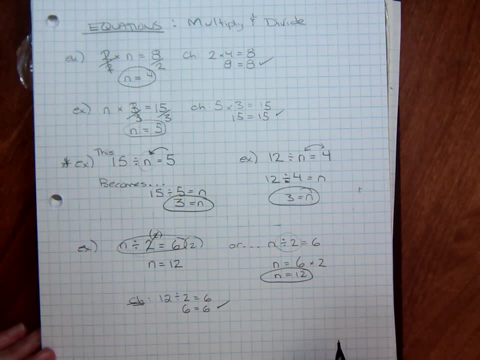 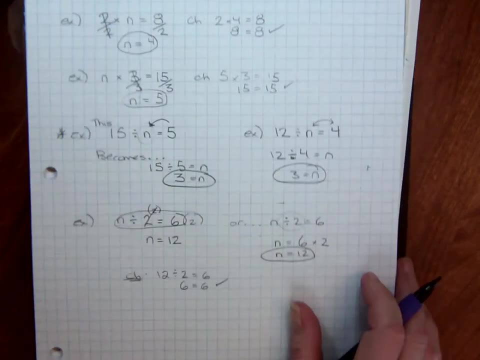 That's how I can check and know that I did it right. Okay, let's go back to our worksheet. Oh, should we do one more? Maybe we should do one more. Let's do one more here. Okay, let's do another example. 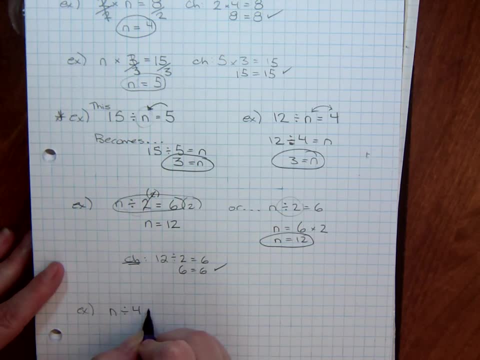 Something divided by 4 equals 2.. Something divided by 4 equals 2.. So that means that I can just times both sides: N equals 2 times 4.. So N equals 8.. Okay, that's what I did. 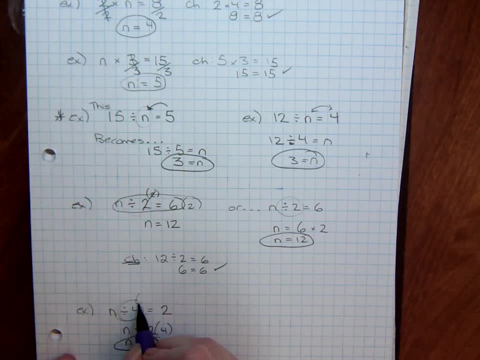 I just took this and I timesed it. I timesed both sides by 4.. These cancel, And 2 times 4 is 8.. And I'll check it: 8 divided by 4 equals 2. It does. 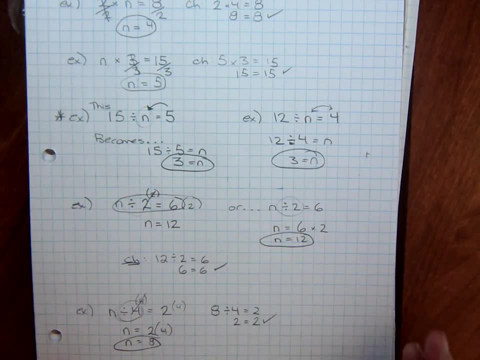 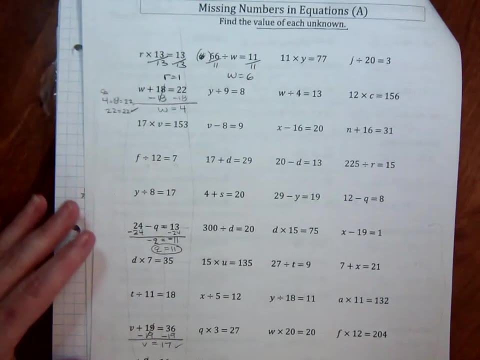 2 does equal 2.. We did it right. Okay, let's go back to our worksheet. So again we're on missing numbers and equations. So let's finish this first column together. Okay, Okay, 17 times something. 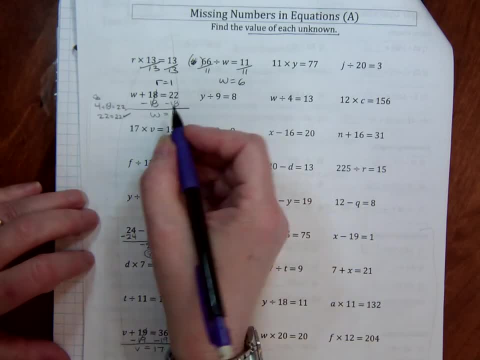 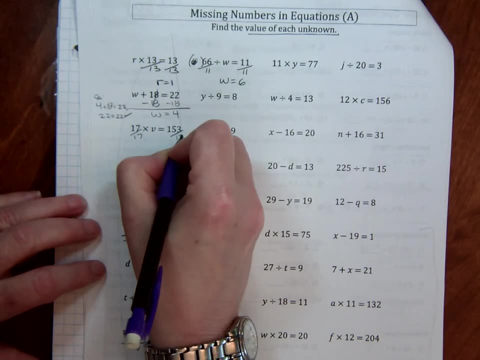 Something is 153.. So since my number's over here and it's not even close to the equal sign, I can divide both sides. Okay, 17 divided by 17 is just 1.. So I'm left with one little v, and that's what I wanted. 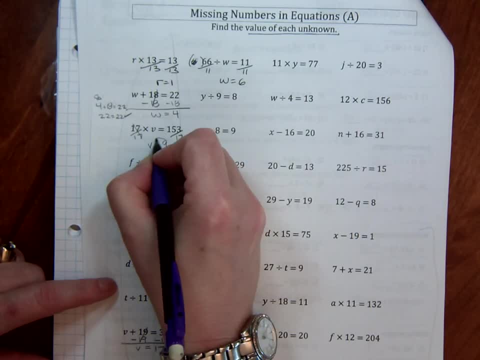 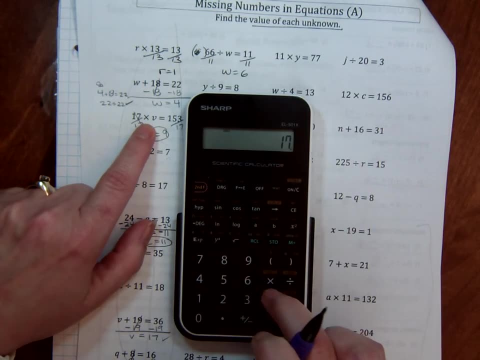 153 divided by 17 is 9.. I can even check it. Let's substitute it in 17 times and I said that v is 9, so I'll check it equals, And it does equal 153. 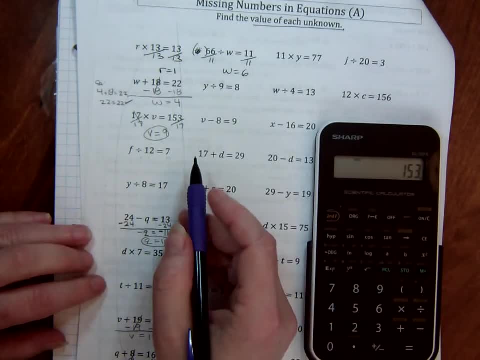 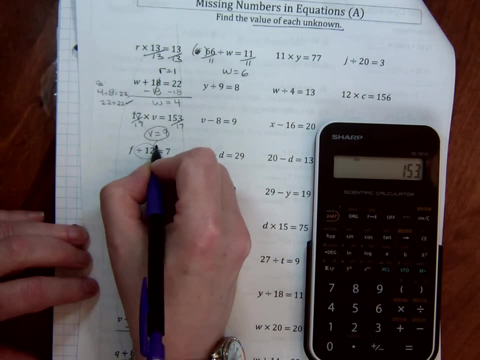 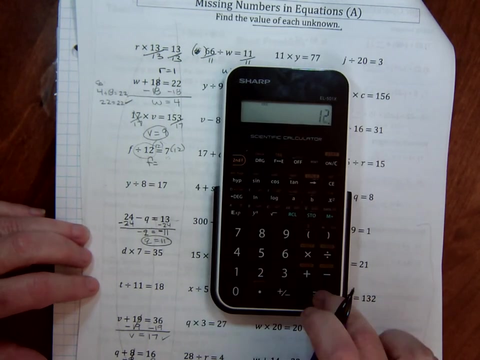 So I know I did it right. Let's move on Something divided by 12 equals 7.. So the opposite of divide is multiply. So I'll multiply both sides by 12.. So f equals 7 times 12, 84.. 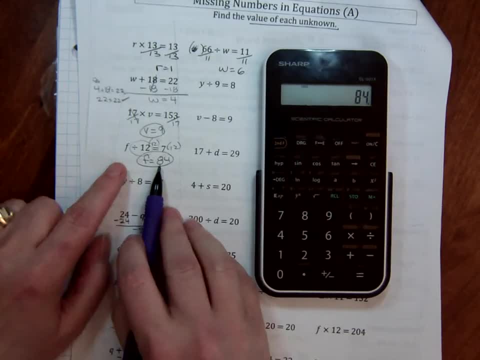 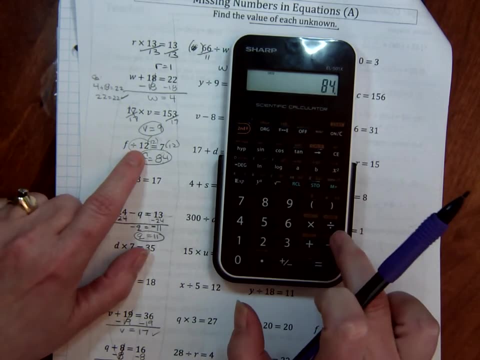 Now if I want to check that, I said that f equals 24. Or 84,, sorry, 84. So 84 divided By 12 should equal 7. And it does. I did it right, Okay. Next one. 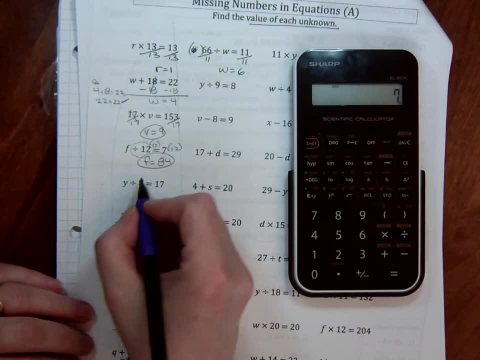 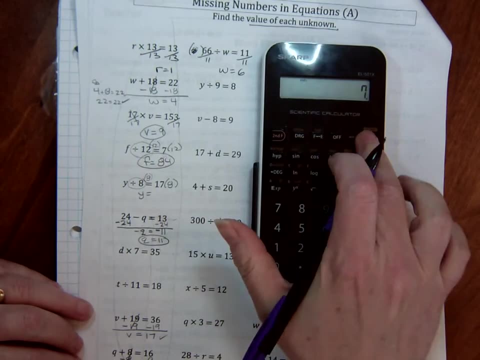 Something divided by 8 equals 17.. So if I times both sides by 8, times both sides by 8, y equals what is 17 times 8? I don't know that. in my head 136.. I'm going to check it. 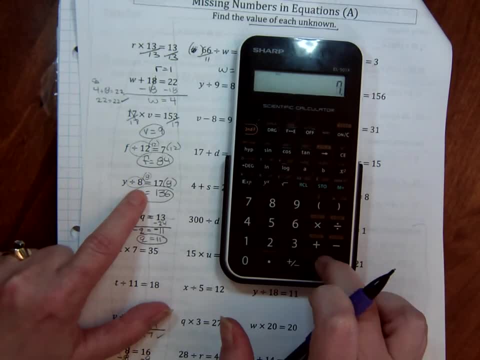 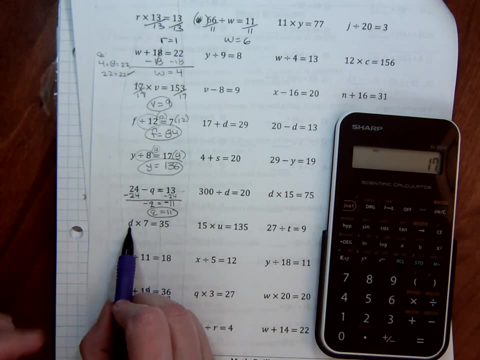 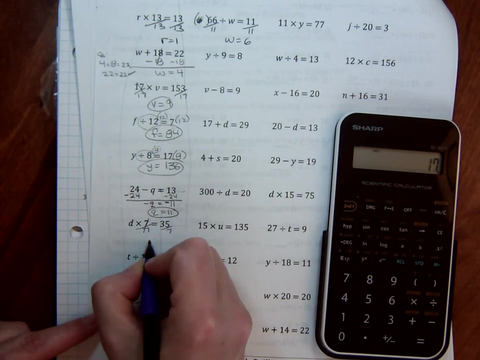 136 divided by 8 should equal 17.. And it does, Okay. Now moving on Something: times 7 equals 35. The opposite of times is divide. Okay, These cancel D is by himself. 35 divided by 7 is 5.. 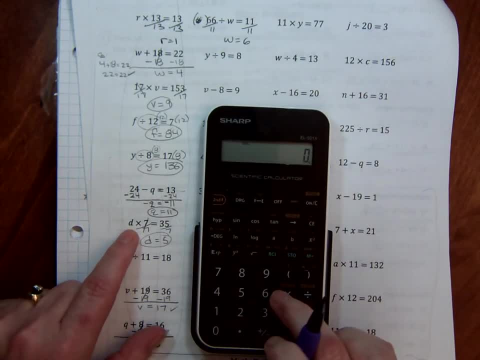 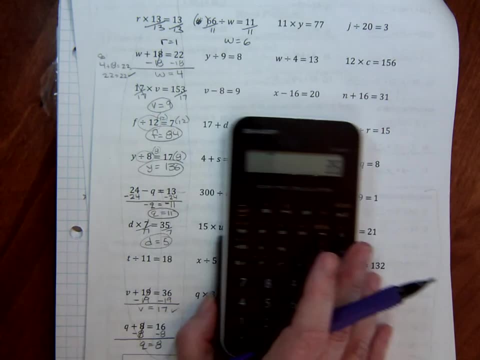 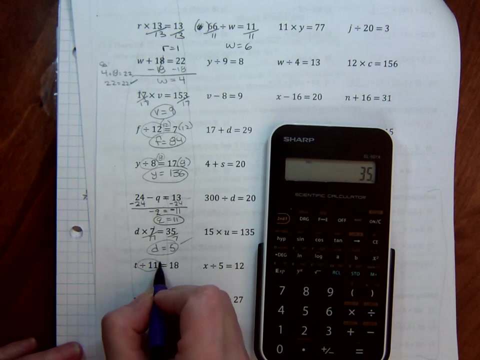 I want to check it. 5, because I said D is 5, substitute it in times 7. It does equal 35. I did it right. Okay, Moving on, Something: divided by 11 equals 18.. The opposite of divide is multiply. 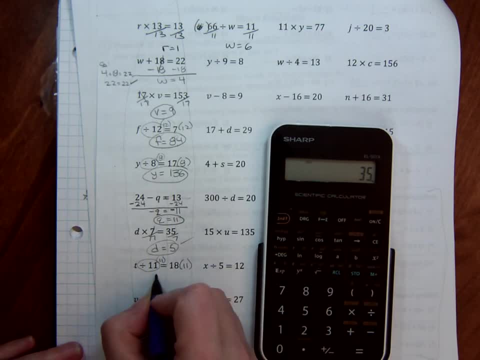 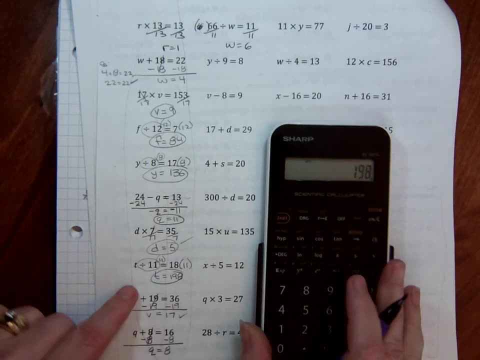 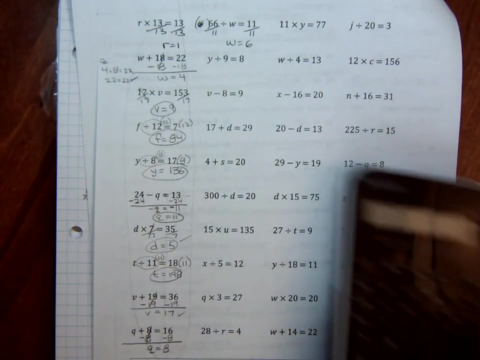 Multiply both sides by 18, or by 11.. T equals 18 times 11, 198.. Check it: 198 divided by 11 should be 18.. And it is Okay. I want you to continue. Finish this page. 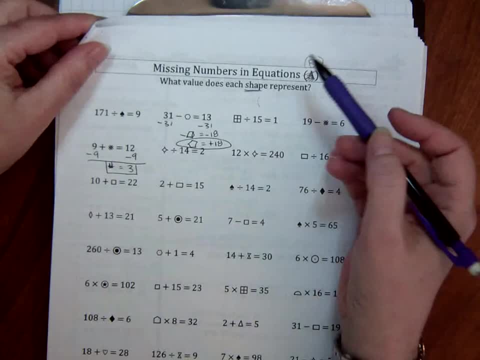 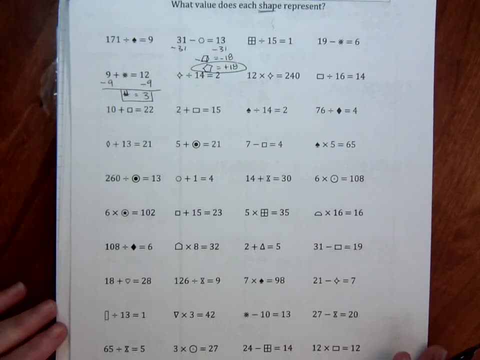 That's part A, And I want you to finish page B. These are the exact same kinds of questions. There is no difference. When you're done all of these, there'll be a small online quiz, something you can do from your phones. 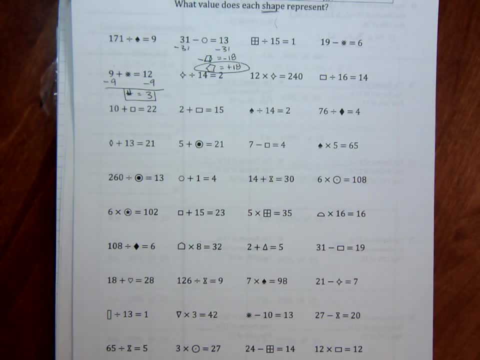 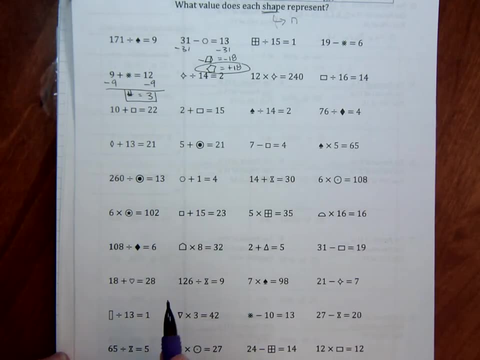 So, again, if you don't have this print out, take a picture of this and write it down. And instead of all these shapes, you could just make each shape, the letter N. You could just make each shape: the letter N, the letter B, the letter M, I don't care.